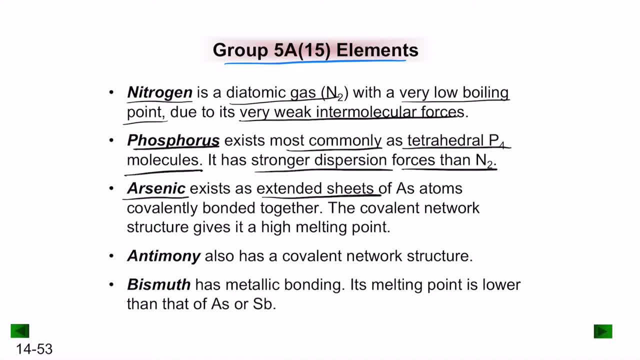 Next we have arsenic. So arsenic exists as extended sheets of arsenic atoms covalently bonded together, and this covalent network structure gives it a really high melting point. Next we have antimony. So antimony also has a covalent network structure. The reason mainly 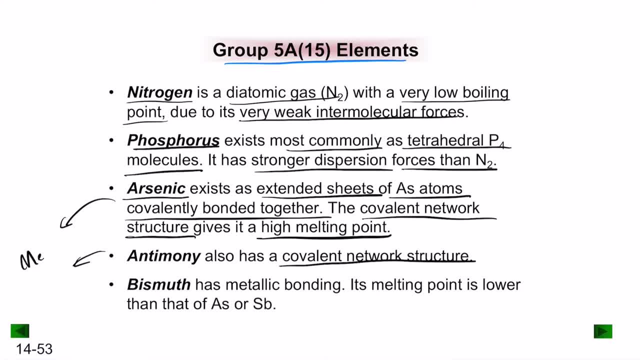 is because arsenic and antimony- both of these- are metalloids, So they are not metals. They are between metals and non-metals. Next we have bismuth. So bismuth has metallic bonding, because bismuth is a metal. 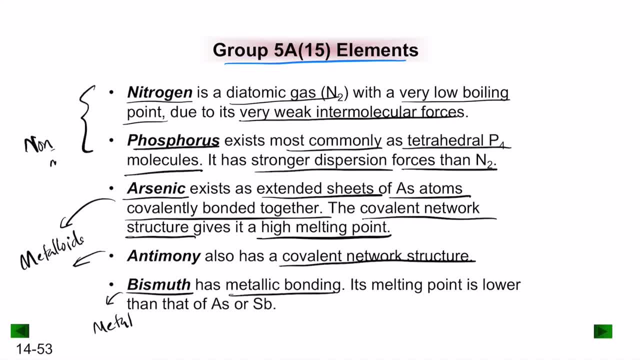 So you have two non-metals, one metalloid and one, two metalloids and one metal. So bismuth also has a. its melting point is generally lower than that of arsenic or lead. So arsenic and antimony. 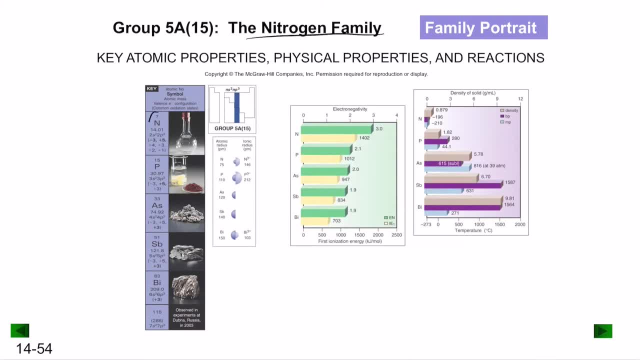 So lets look at the five group elements to the Nitrogen family. So we start with nitrogen, posperous arsenic, antimony, bismuth, And you already know that the electronic configuration is NS2, MP3.. So this is the general electronic configuration for all group five elements. 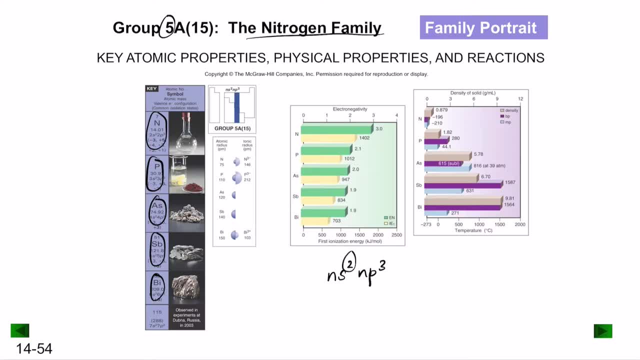 So the group number itself tells you the number of valence electrons. So the number of valence electrons is five. So that gives you the group five elements group number. and you already know the electro negativity is highest for, highest for nitrogen and as you come down the group it automatically decreases. 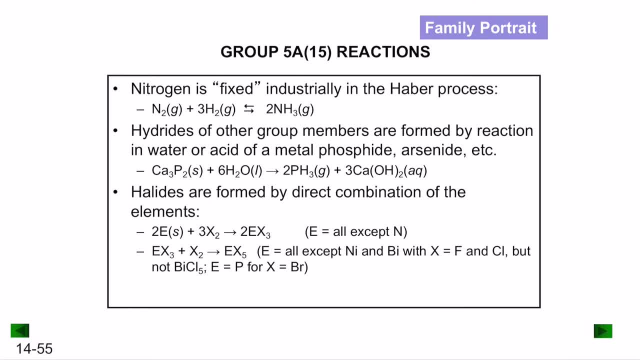 so what are the common reactions that we can see? so generally? a nitrogen is fixed industrially in the Hibbert process so it's used to used in the production of ammonia, which is generally used in different different processes as fertilizer, as the coolant. so there are multiple purposes that are being used. 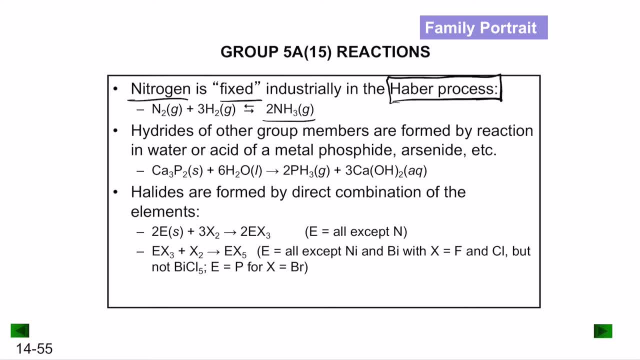 and the that process is generally done by the hipers process, which we will discuss in the contending the lectures as we go on. next we have hydrates of other group members are generally formed by reactions in water or acid of a metal, phosphide, arsenide, etc. so, for example, calcium phosphide reacts with 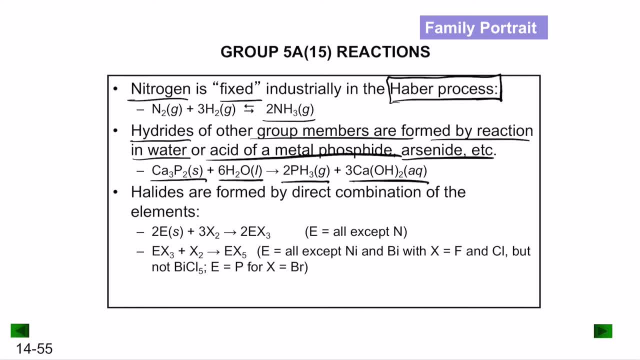 water to form phosphine and calcium hydroxide, so a purple phosphate hydride and calcium hydroxide. so halides are generally formed by direct combination of these elements. so when you combine directly with the hydrogen hydrogen, that is the process you are going to see. 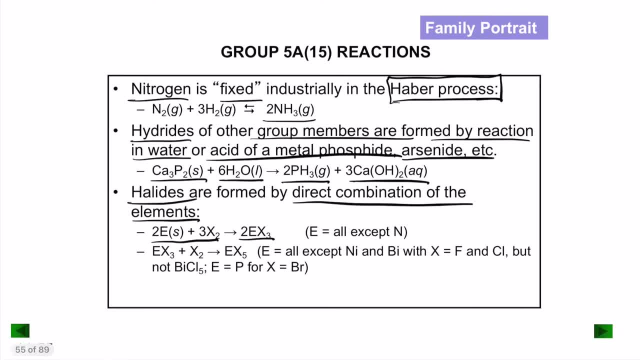 so the combination directly will result in the formation of ex3, except for nitrogen. ex3 in in combination with another x2 results in ex5. so you start with a smaller halide to a larger halide as you mix them, more and more quantities. so this happens except with nickel and bismuth. 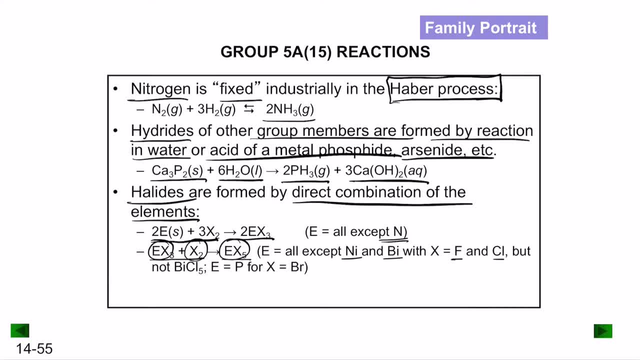 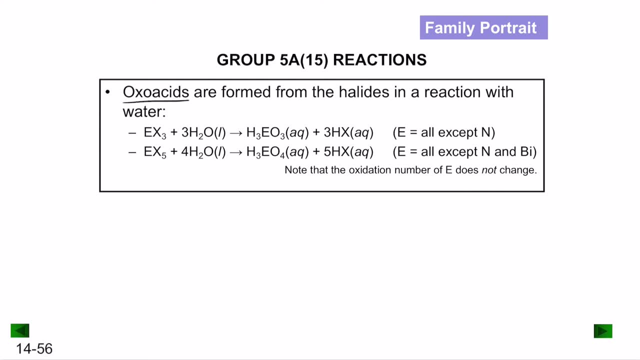 and it generally happens with fluoride, fluoride and chloride, and it generally does not create bismuth. so bismuth cl5 will not be, so bi cl5 will not be occurring. so e, here will be px, here will be bromide. next we have what we call oxo acids. so oxo acids are formed when you have halides in. 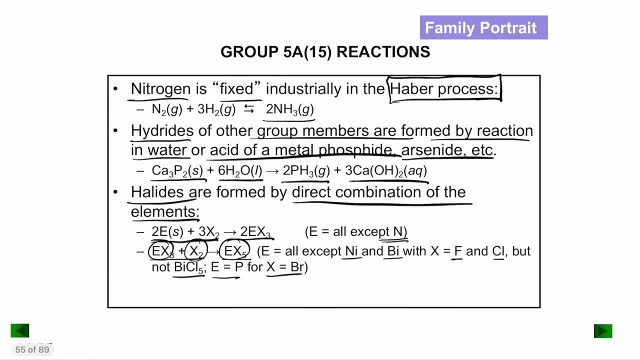 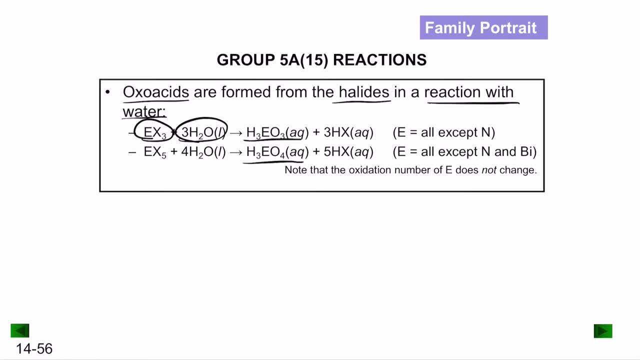 a reaction with water. so you are already creating the halides. so the halides that you have created here with the group 5 elements, when you mix them in water, that results in the formation of oxo acids. so this oxo acids are really powerful acids and these are the common acids that you would generally see in a different group purposes. so these are sometimes weak acids, sometimes strong acids. an example of this would be to take hno3, which results in the nitric acid. you have hno2, which is nitrous acid. you also have phosphoric acid, so h3po3 and h3po4- phosphorous acid and phosphoric acid. so these are the common. 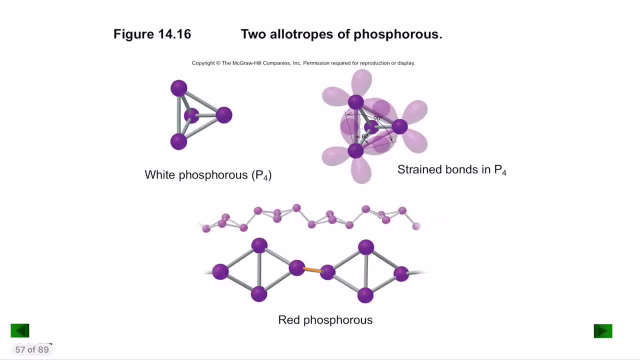 acids that you will generally see in the production from group 5 reactions. now, phosphorus can be found in different versions. one of them is whitepasparous, so whitepasparous has a strained bond, so that's why most more common form of phosphorus is dotpospous. closing ere use is big mashup. 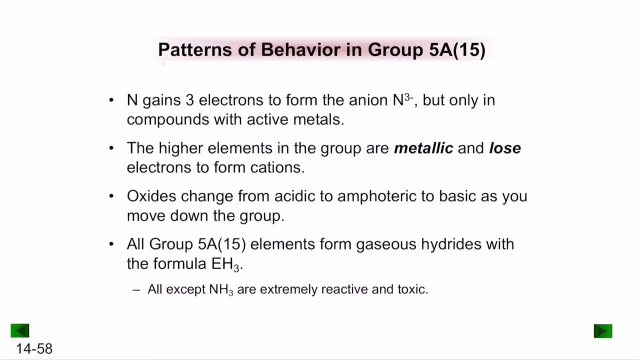 matrix. now let's look at the patterns of behavior in group 5a, group elements. so nitrogen gains three electrons to form the anion n3-, but only in compounds with active complexル. anion andBER course is Xiaoying. we base on early en来. 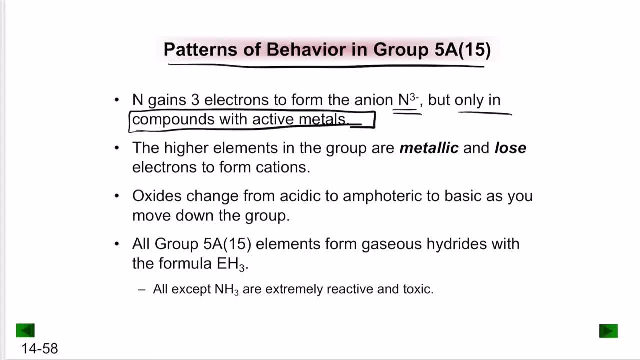 active metals. remember this part that nitrogen only does this when it is in compounds with active metals. next, the highest elements in the group are generally metallic and are ready to lose electrons to form cations. so oxides generally change from acidic to amphoteric to basic as you move down. 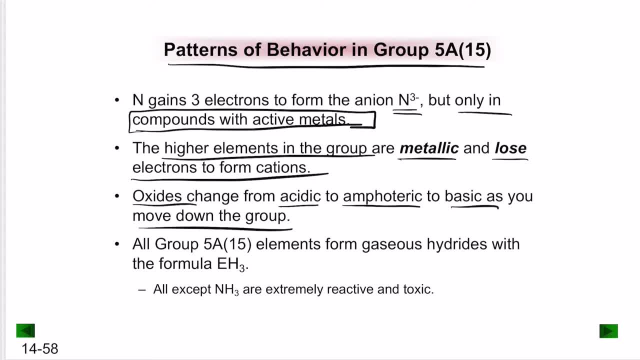 the group. so nitric, as nitric oxide is generally acidic, you go into phosphorus, phosphorus oxides, which are generally amphoteric, finally towards basic, where you end up with bismuth. next, all group 5a elements form gaseous hydrides with the formula eh3. all except nh3 are extremely toxic and 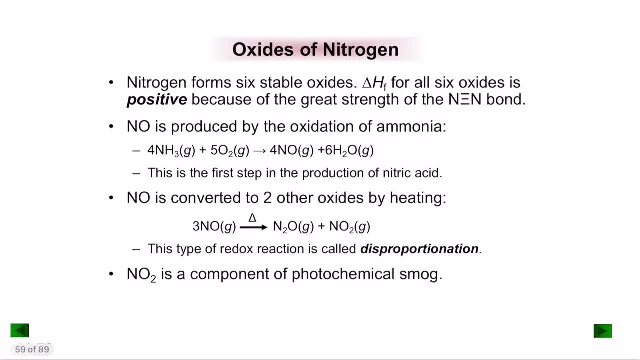 extremely reactive and toxic. next you have oxides of nitrogen. so nitrogen can form six stable oxides and the enthalpy of formation of all the six oxides is positive because of the great strength of the triple bonded nitrogen. now, nitrous oxide no is produced by the oxidation of ammonia. so 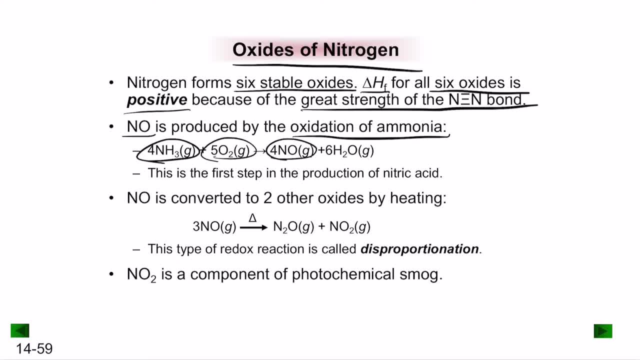 when you take ammonia and oxidize it in the presence of oxygen, it undergoes the formation of nitrous monol, nitrogen oxide, and this is nitrogen monoxide. this is the first step in the preparation of nitric acid. so this is the first step where we 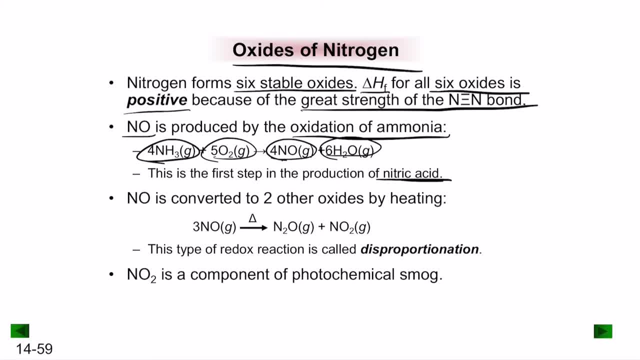 in production of nitric acid, where we first create nitrogen monoxide. now this nitrogen monoxide is converted to two other oxides when you heat it. so when you heat nitrogen monoxide it becomes dinitrogen monoxide and nitrogen. dioxide. now this type of redox reaction, where both the elements 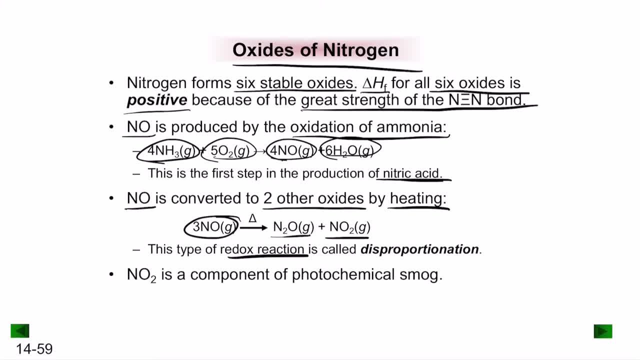 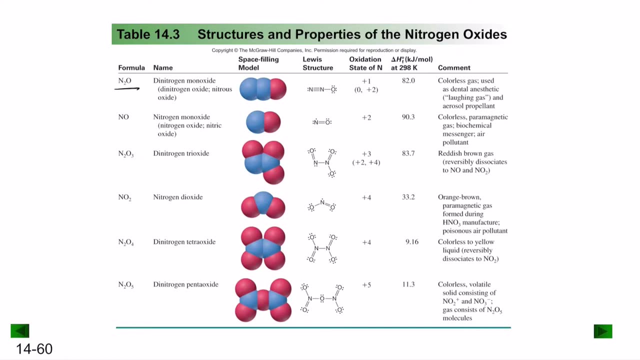 are generally taken into consideration and both of them, one undergoes reduction and the other undergoes oxidation- is called as disproportionation reaction, and this no2 is the component of photochemical smog. so these are the six forms of nitrogen oxides. you have dinitrogen monoxide, nitrogen monoxide. 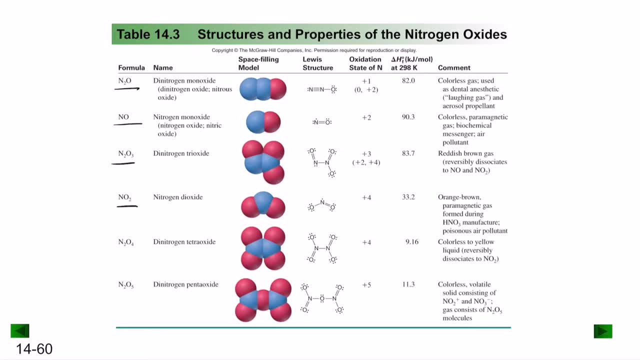 dinitrogen trioxide, nitrogen dioxide, dinitrogen tetroxide and dinitrogen pentoxide. so now, dinitrogen monoxide is a colorless gas and is generally used as a dental and dental anesthetic, most commonly known as laughing gas, and it is also an aerosol- aerosol propellant. 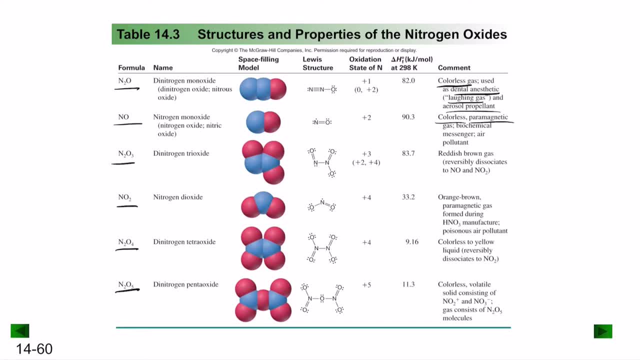 you have nitrogen monoxide, which is generally colorless, paramagnetic gas and is a biochemical messenger and an air pollutant. you have dinitrogen trioxide, which is a reddish brown gas which undergoes reversible dissociation to form both nitrogen monoxide and dinitrogen dioxide. so 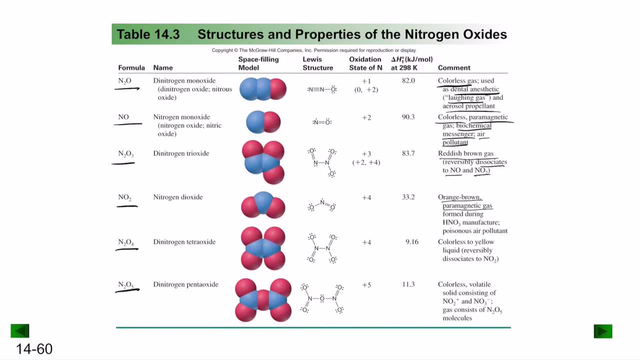 nitrogen dioxide is an orange brown gas with parametric, so it's also paramagnetic and it generally formed during the production of nitric acid and it is also a poisonous air pollutant. you have dinitrogen tetroxide, which is colorless to yellow liquid and it generally 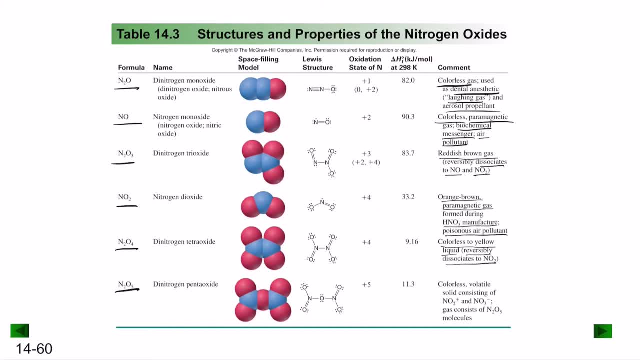 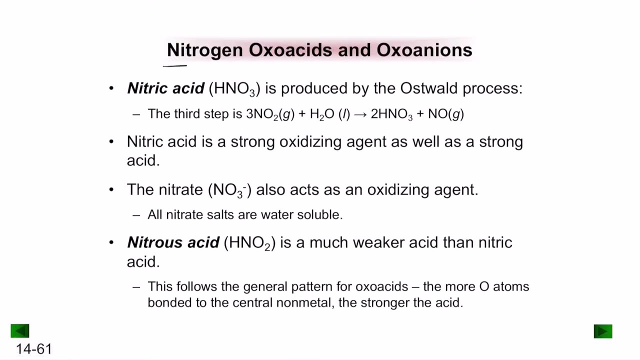 dissociates to nitrogen dioxide. you have dinitrogen pentoxide, which is a colorless, volatile solid consisting of nitrogen dioxide and NO3, and this consists of the gas. consists of N2O5 molecules. now let's talk about nitrogen, oxo acids and oxo anions. now nitric acid HNO3 is produced. 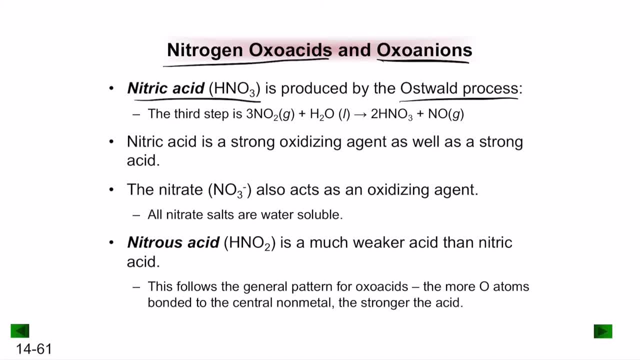 by the process which we can generally call the Oswald process. so Oswald process uses the step, the nitrogen dioxide, and mixes it with water to produce nitric acid and nitrogen monoxide. and nitric acid. here is a really strong oxidizing agent as well as a really strong acid, and the ion that it produces, the nitrate, also acts as 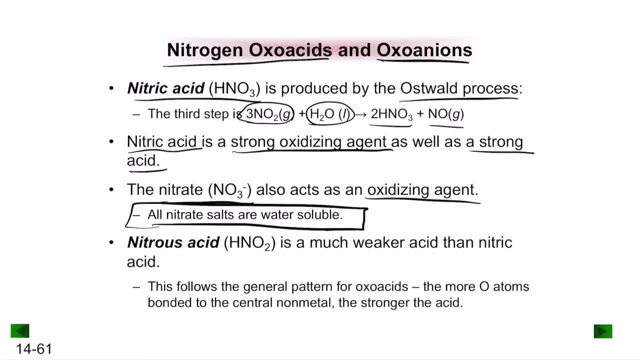 an oxidizing agent and all nitrate salts are water soluble because of the presence of the ions there, the oxygen there. next you have nitrous acid, which is HNO2, which is a much weaker acid than nitric acid HNO3.. and this generally follows a pattern of oxo acids: the more oxygen atoms bonded to the 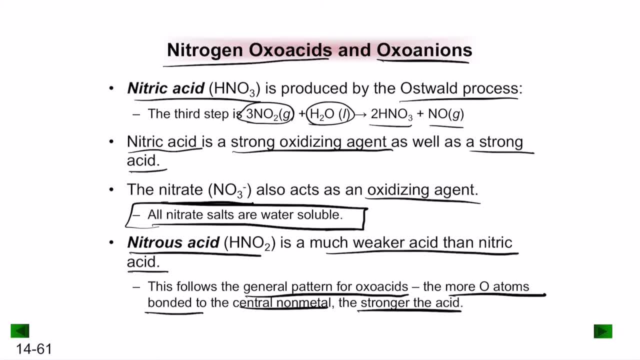 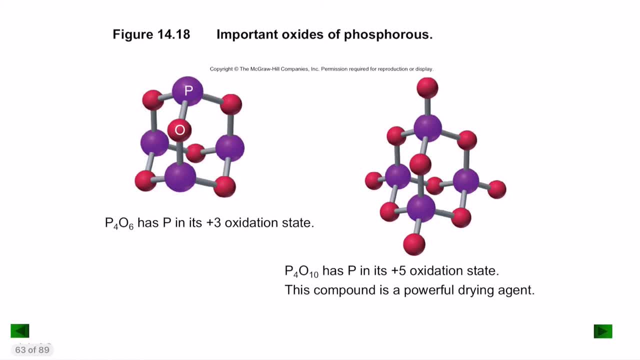 central nonmetal, the stronger the acid. so remember this principle, that the more the oxygen atoms, the more stronger the acid. so next important phosphorous oxides, you have P4O6 and P4O10. so P4O6 has the phosphorous in plus 3 oxidation state and P4O10 has the 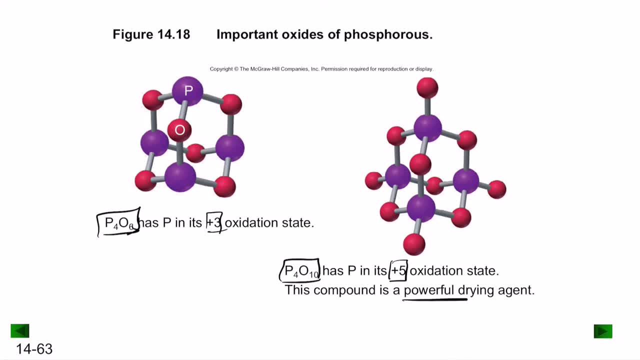 phosphorous in plus 5 oxidation state and P4O10 is generally used as a powerful oxidizer. P4O10 is generally used as a powerful oxidizer. P4O10 is generally used as a powerful drying agent in most commonly in most commonly in. 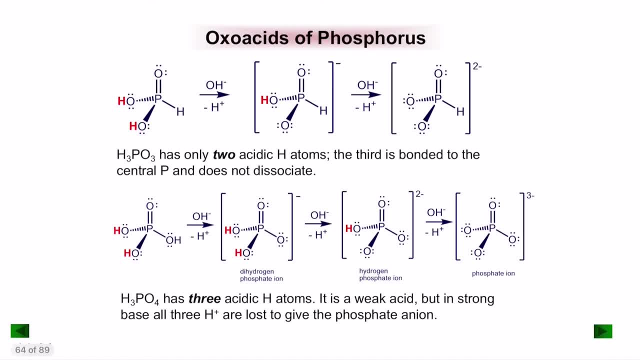 dry washing You have oxo acids of phosphorus. so the first one is H3PO3, which is phosphorous acid, only has two acidic hydrogen atoms. so there are only two acidic hydrogen atoms. and the third is bonded to the central phosphorus and does not dissociate. so this one does not dissociate. 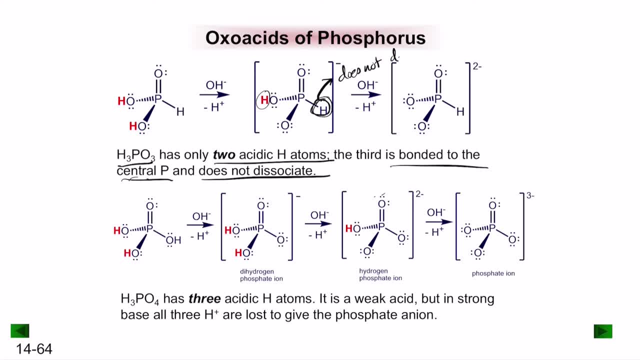 so this one does not dissociate. So the only ones that dissociate are the ones bonded to the oxygen. the rest will not dissociate. You have H3PO4, which is phosphoric acid, contains three acidic hydrogen atoms. so these are the three acidic hydrogen atoms and it is also a weak acid, but in strong basis- all three. 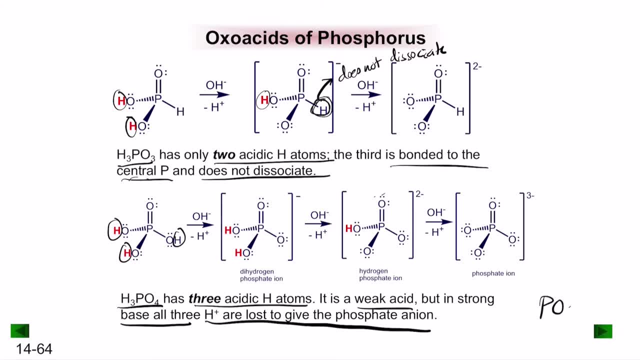 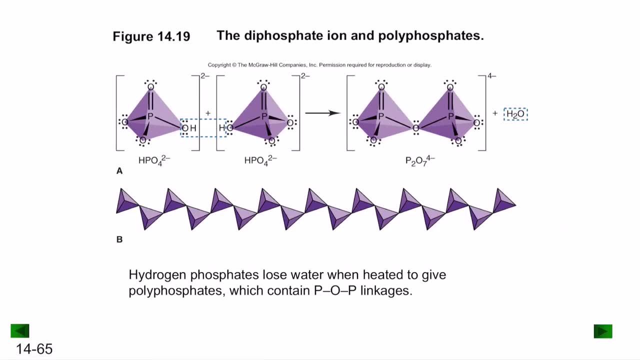 hydrogens are lost to give you the phosphate anion, so phosphate anion is PO4 3-. Next, you have the diposipate ion and polyphosphate, so diposipate ion is HPO4 2- and this, under further dissociation, results in the production of P2O7 4- and this is the what we call the. 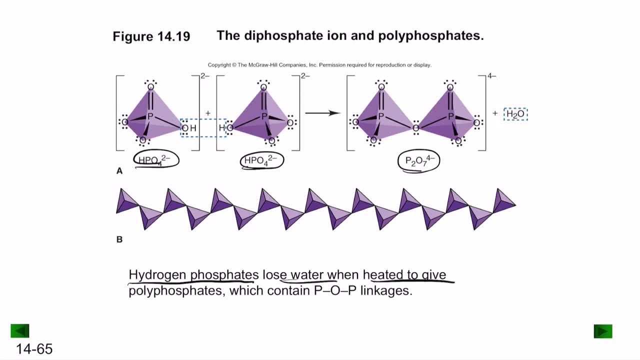 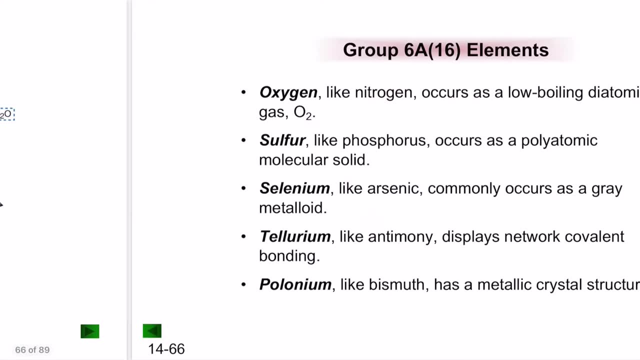 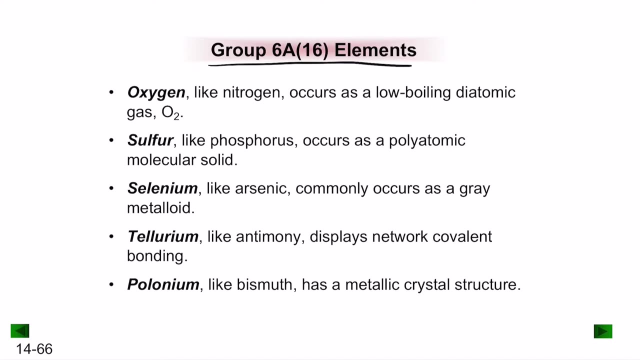 hydrogen phosphates. these generally lose water when heated to give polyphosphates which contain the linkage phosphate, oxygen, phosphate linkage, so POP linkage. Next we have group 6A elements. let us go into group 6. so group 6 contains oxygen, sulfur, selenium, tellurium and polonium. 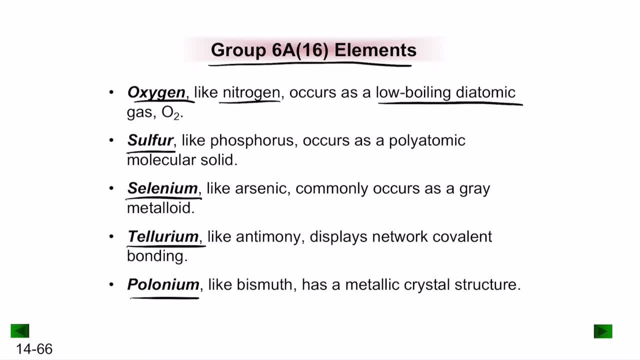 So oxygen, like nitrogen, occurs at a low boiling point- It is a low boiling diatomic gas. and sulfur, like phosphorus, occurs as a polyatomic molecular solid. selenium, like arsenic, commonly occurs as a gray metalloid. tellurium, like antimony, displays a network covalent bonding. and finally, polonium, like bismuth, has a metallic crystal. 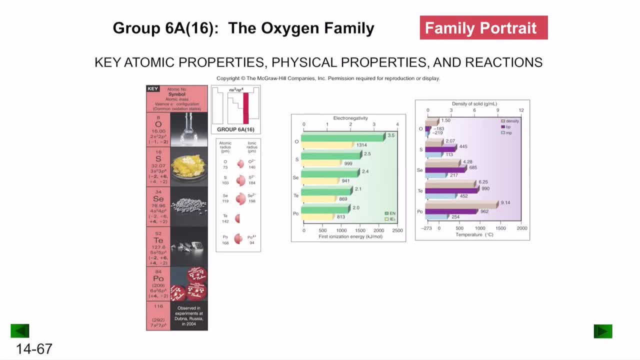 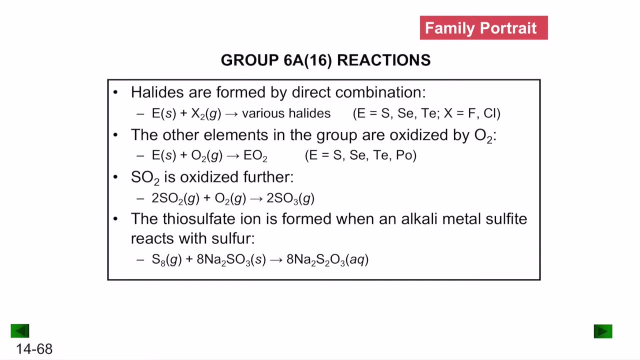 structure. so these are the group 6A elements and their general electronic configuration is NS2NP4.. Next let us talk about the common reactions of group 6A elements. so halides are generally found by direct combination. So when you mix a halide with the solidic materials, generally sulfur and selenium, they 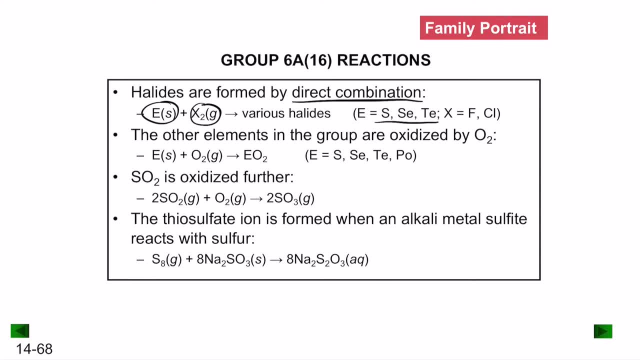 generally produce various halides, So most commonly, sulfur, selenium and tellurium are the common ones that produce halides, and the halogens that are generally mixed are either fluoride or chloride. Next, what are the other elements? are generally oxidized by oxygen, so this is resulting in 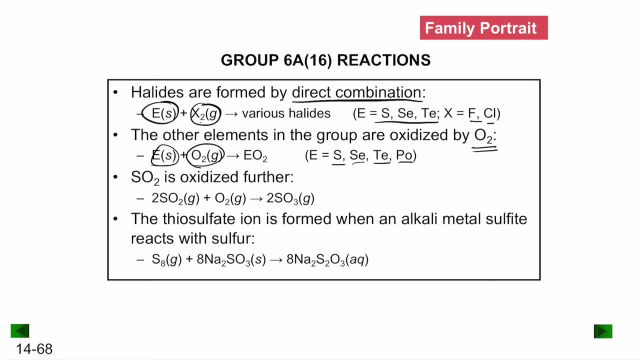 the formation of all the other ones: sulfur, selenium, tellurium and polonium all form oxides with oxygen. Next, sulfur dioxide is generally further oxidized to form sulfur trioxide, resulting in the formation of sulfur trioxide. Next, the thiosulphate ion is found when you have an alkali metal, sulphate, reacting with. 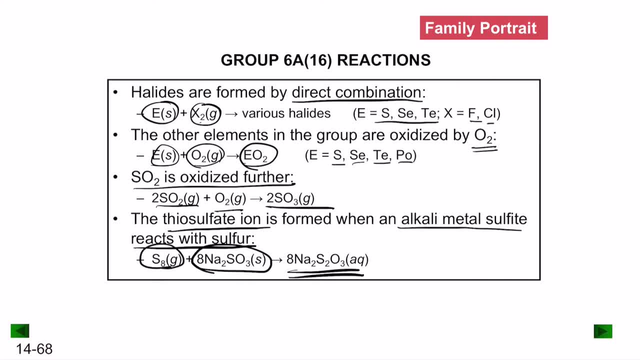 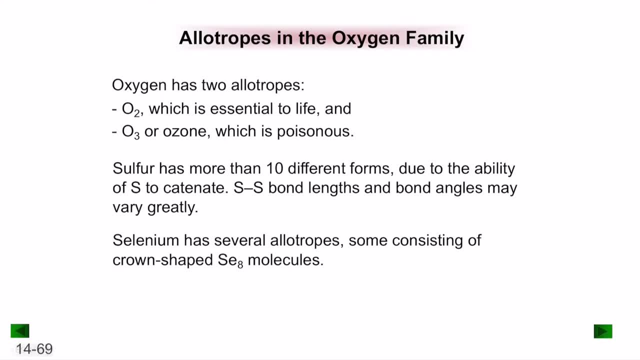 sulfur. so alkali metal sulphate, when it reacts with a acid form of sulfur, results in the formation of thiodium alkali metal sulphate. so this is the formation here. Next, let us talk about allotropes in the oxygen family. Oxygen has two main allotropes: O2, which is essential for life. 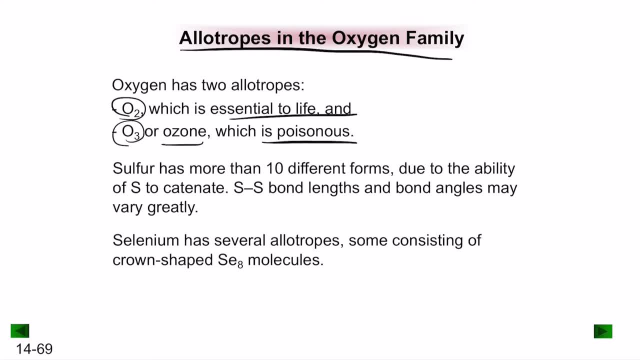 And O3 or ozone, is basicallyna robotic carbonene Exactly, which is generally a poisonous gas. Now, sulfur has more than 10 different forms and, due to the ability to sulfur to catenate- remember the term- catenate represents that it can bond to itself. 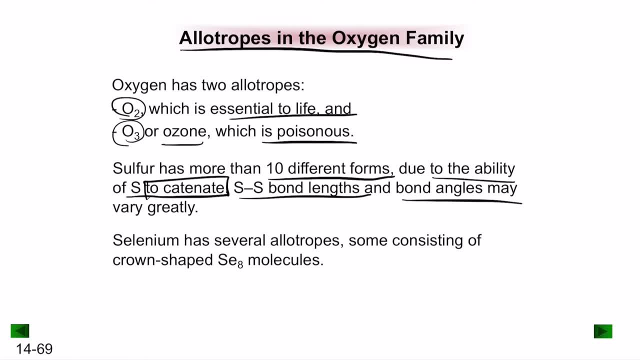 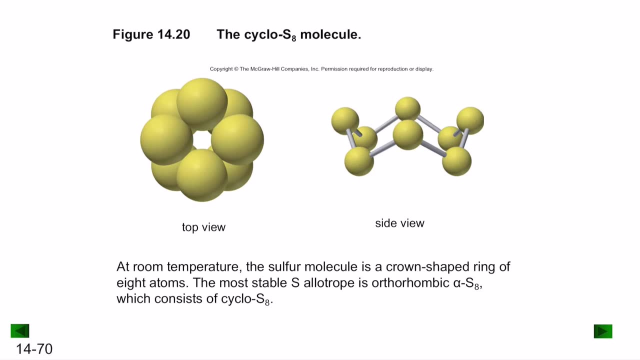 and this sulfur-sulfur bond lengths and the bond angles may vary greatly. Now, selenium has several allotropes and some consisting of crown shaped seleniumate molecules. Now this is an example of the cycloacet molecule, in the top view and the side view At room temperature, the sulfate molecule. 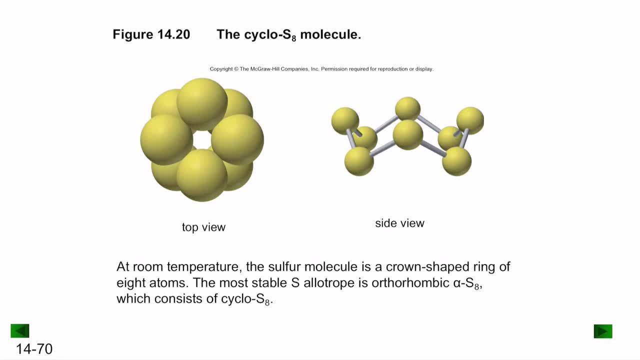 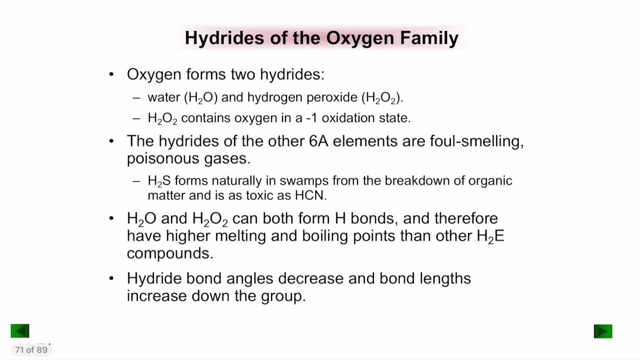 is a crown shaped ring with eight atoms, and the most stable sulfate is the orthorhombic alpha acetate. So this is the one which consists of cycloacetate. Next, let's talk about hydrides of the oxygen family. So we already know the two common hydrides of the oxygen family. one is water. 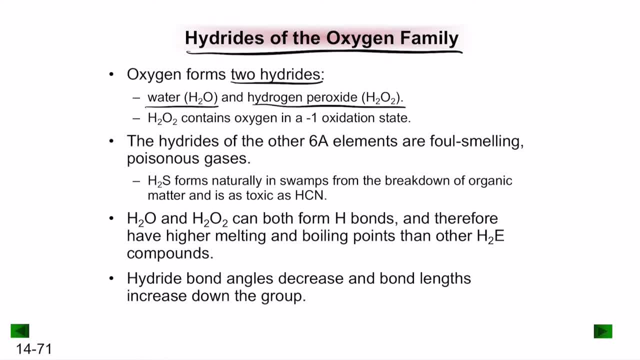 H2O and hydrogen peroxide H2O2.. So water has oxygen in its regular state, but oxygen H2O2 is the hydrogen peroxide H2O2.. So water has oxygen in its regular state, but oxygen H2O2 is. 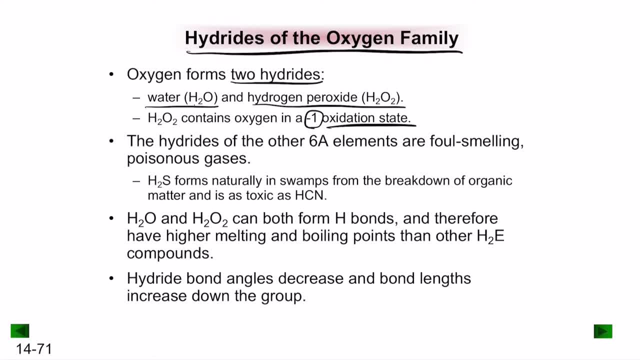 H2O2 has an oxygen in negative one oxidation state and the hydrides of all the other 6A elements are generally foul smelling poisonous gases. For example, H2S forms naturally in swamps and the breakdown of organic matter and it's similar to the toxicity of higher cyanide, cyanic acid and 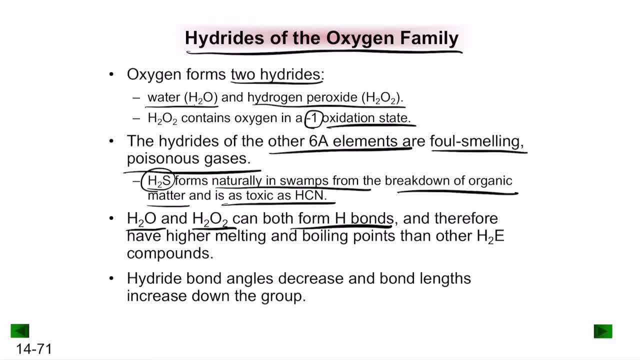 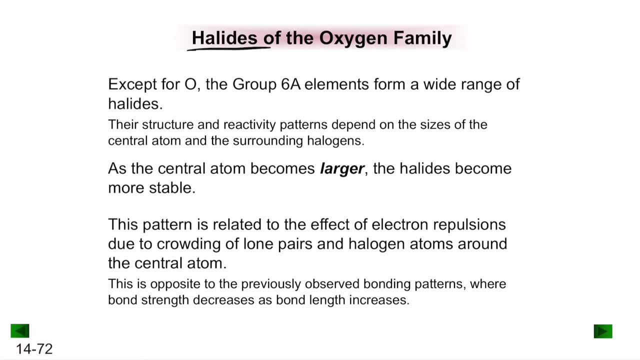 H2O and H2O2 have both hydrogen bonds, therefore have higher melting and boiling points in comparison to all other compounds of the 6A group elements. and this hydride bond angles decrease and the bond lengths increase down the group. Next let's go to the halides of the oxygen. 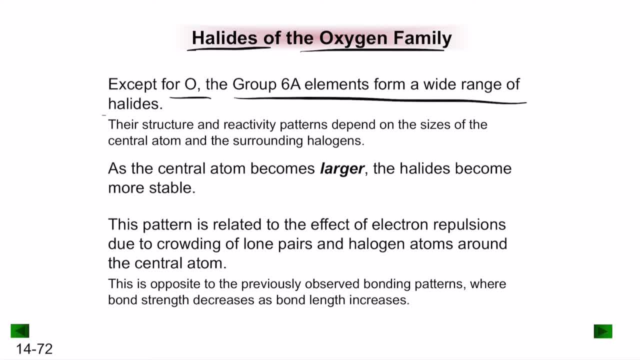 family. Except for oxygen, all the group 6A elements have wide range of halides and as the central atom becomes larger, the halides become more stable. So this pattern is related to common the effect of electron repulsions due to the crowding of lone pairs and the halogen atoms around the central atom. 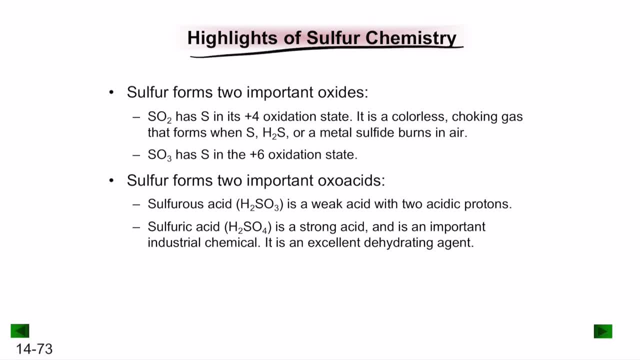 Let's talk about the highlights of the sulfur chemistry now. So sulfur has two main important oxides: sulfur dioxide and sulfur dioxide. So sulfur dioxide has two main important oxides: sulfur dioxide and sulfur dioxide. dioxide and sulfur trioxide. so sulfur dioxide has sulfur in the plus four oxidation state. 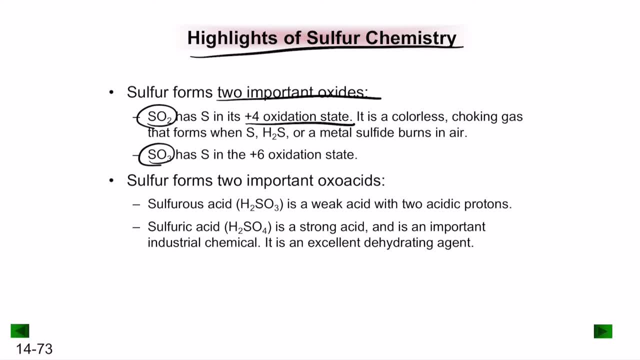 and sulfur trioxide has the sulfur in plus six oxidation state. it is a colorless. sulfur dioxide is a colorless choking gas that forms when sulfur, h2s or a metal, sulfide, burns in air. let's next. sulfur has two important oxo acids. so sulfur has two forms, two important 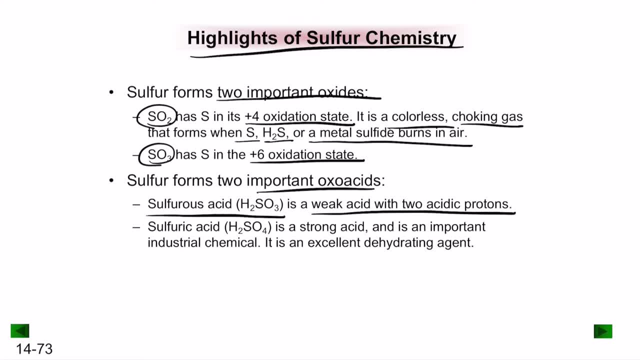 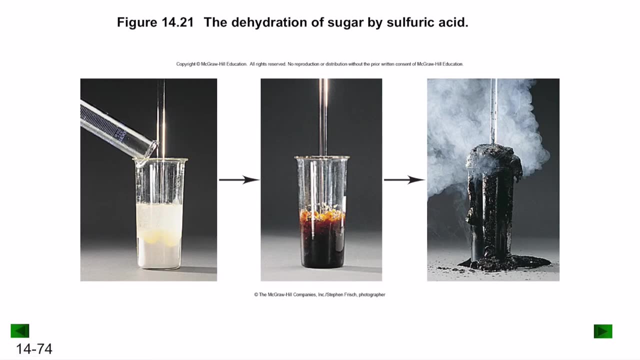 oxo acids. so sulfurous acid, which is a weak acid with two acidic protons, and sulfuric acid is a strong acid and is an important industrial chemical and it's generally an excellent dehydrating agent. now the dehydration of sugar by sulfuric acid. this is the reaction. 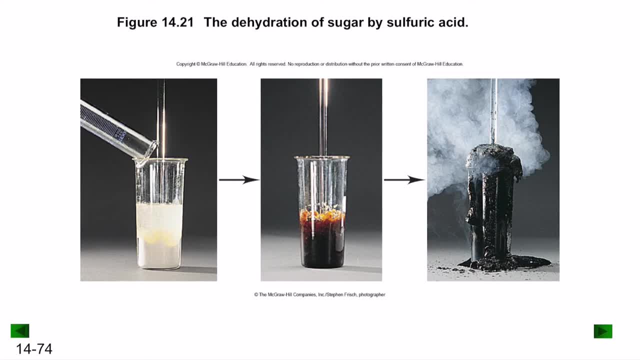 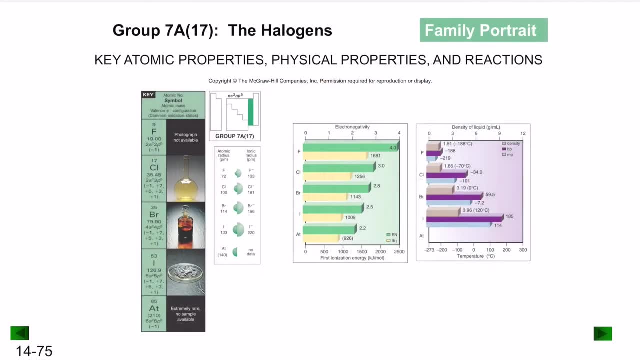 that it shows. so when you pour sulfuric acid into sugar, it results in the dehydration, where it removes water from the glucose, resulting in the formation of. so let's get into the fire. so this is the penultimate group group. seven, eight group elements, so commonly known as: 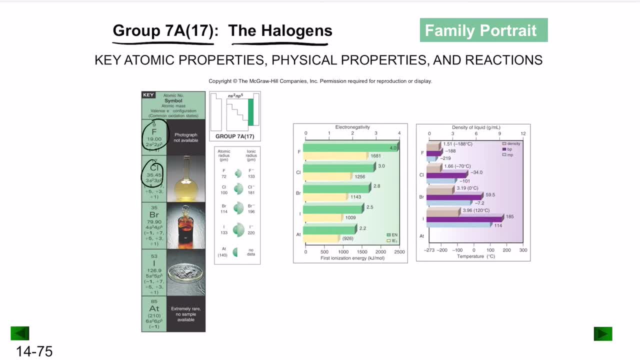 the halogens. so these are elements that involve fluorine, chlorine, bromine, iodine and atrium. so this final element is something that is not used very often and this element is generally extremely rare, so we do not use that element often, so we are going to focus more on these. 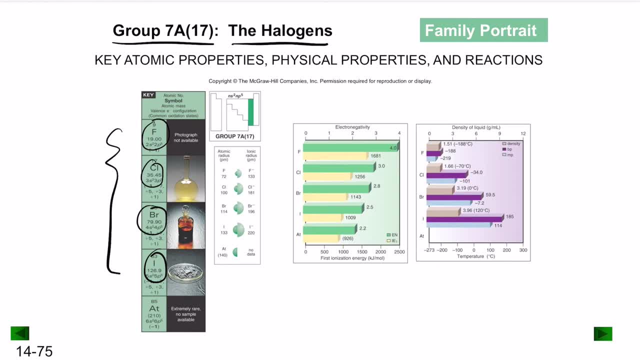 four elements: fluorine, chromine, chlorine, bromine and iodine, because they are more abundant. now, as you already know, because it is the seven a group elements, they have the electronic configuration ns2 and b5 and their electronegativity you start with. they have one of the highest amounts. 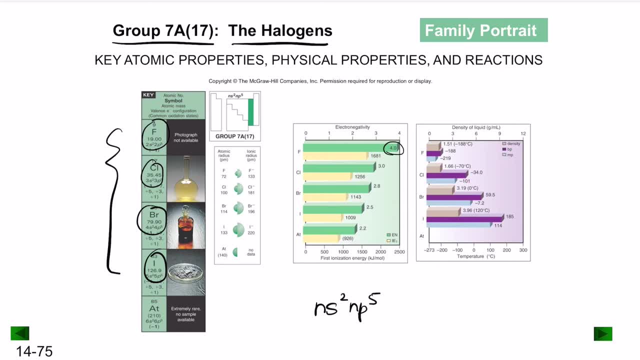 of electronegativity in all the periods of elements. so in every period the. these elements generally have the highest amount of electronegativity, with fluorine having the highest amount of four on the Pauling's electronegativity scale, and as the size increases automatically, the 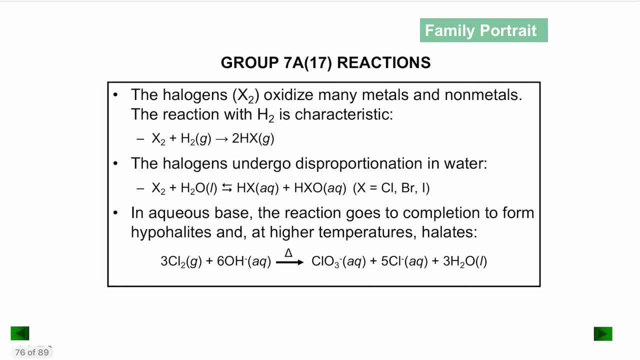 density also will increase with along the group. So let's talk about some of the reactions. so the halogens generally oxidize many metals and nonmetals and the reaction with hydrogen is characteristic. so you have hydrogen mixing with the halogen, resulting in the formation of hydrohalic acid and hydrogen also undergo. 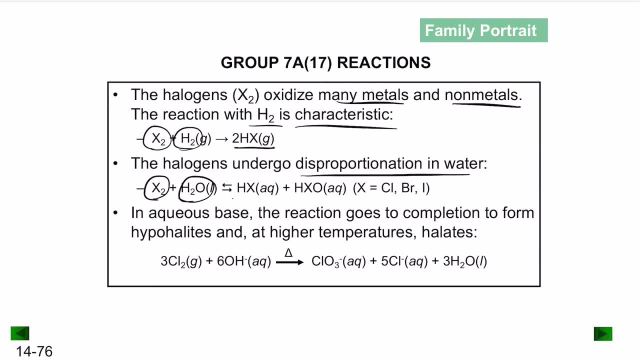 disproportion reaction in water. when you mix them in water it produces the acid plus the oxo acid formation as well. now in aqueous base the reaction goes to completion to form hypo halides And, at higher temperatures, halides, So hypo halides resulting in the formation of ClO3 minus and halides at higher temperatures. 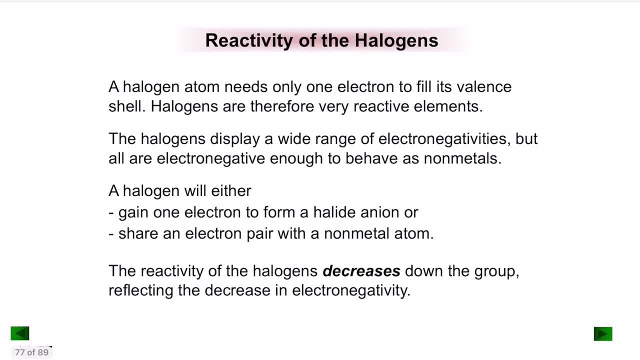 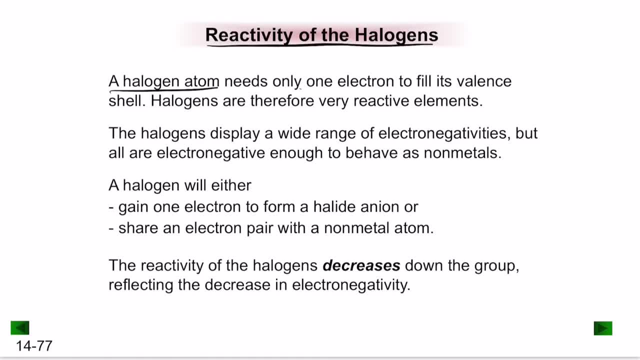 So halides are the molecules ClO3 generally forms at higher temperatures. Next let's talk about the reactivity of halogens. so a simple halogen atom only needs one electron to fill its valence shell because it has the configuration ns2 and b5, so it only needs 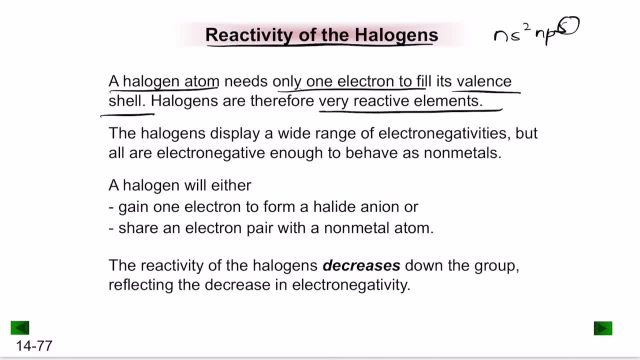 one electron to fill its valence shell. So which means that these elements are Generally very reactive and the halogens Generally display a wide range of display a wide range of electronegativity, but are all electronegative enough? behaviors, nonmetals, a halogen. 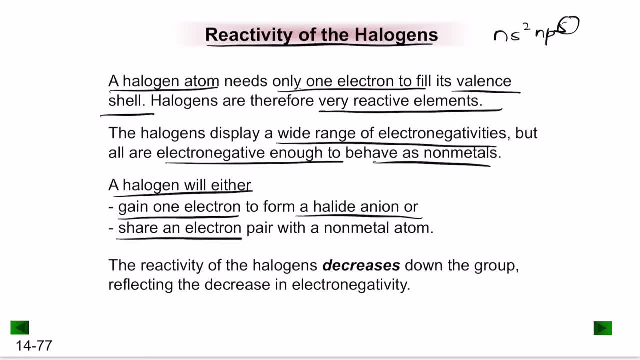 will either gain one electron from a halide ion or share an electron to whether nonmetal, so either resulting in the formation of an ionic bond or in the formation of a covalent bond. So, with an element that donates an electron, It becomes an ion, alteon. 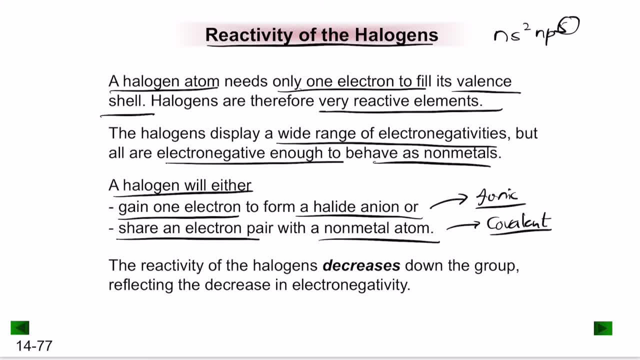 So with an element that donates an electron, it becomes on an ION. So with the element, So with an element With the elements Donates an electron to, does not element, which generally takes an electron, so it shares an electron and forms a covalent. 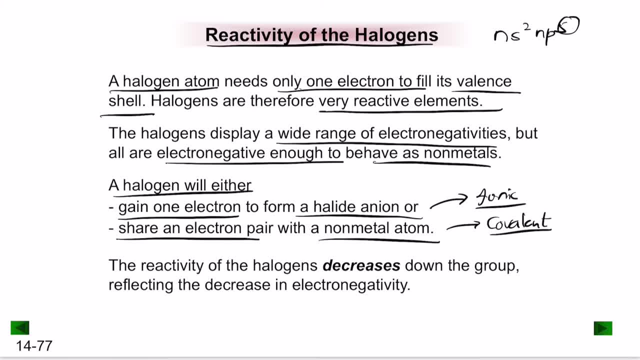 bond. So an example of this to look at, for example, the formation of: so mostly with metals, mostly with active metals, it results in the formation of an ionic substance. and mostly with, mostly with nonmetals, it results in the formation of a covalent molecule. 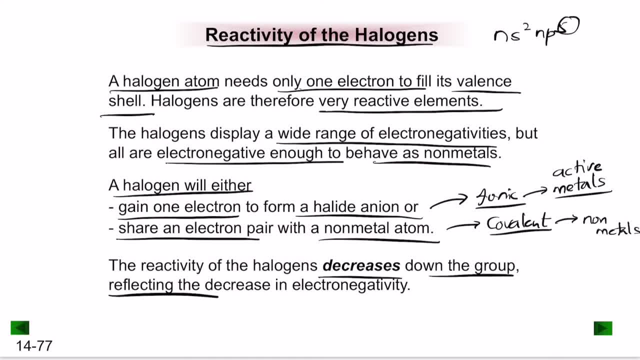 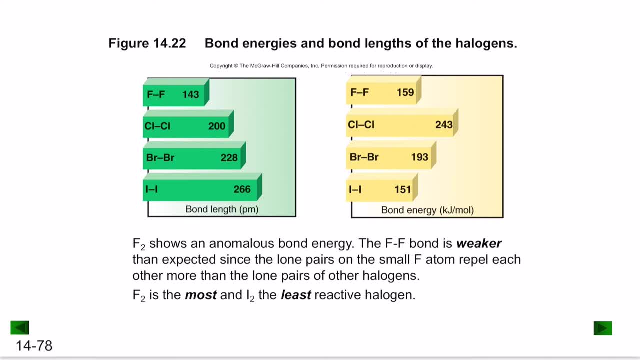 Now the reactivity we have had decreases down the group and reflecting the decrease in the electronegativity. So let's look at the common bond energies of the elements. So fluorine-fluorine has a bond energy of 143, chlorine-chlorine 200,, 228 to 266.. 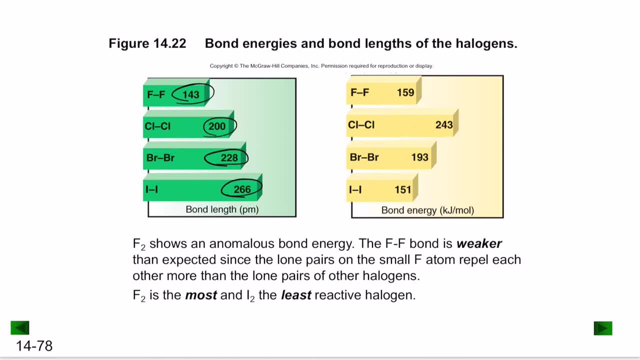 The reason for this increase is this size and when you look at the bond energies you notice something different is that fluorine-fluorine generally has a little lesser bond energy in comparison to chlorine-chlorine, and bromine-bromine and iodine-iodine generally have lesser bond energies in comparison to chlorine-chlorine. 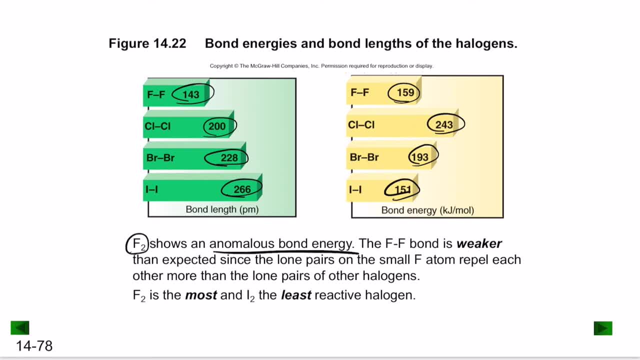 So fluorine is the only one that shows an anomalous bond energy. The reason is because the lone pairs on the small fluorines- fluorine atoms, repel each other more than the lone pairs on the other halogens, and this fluorine is the most. and 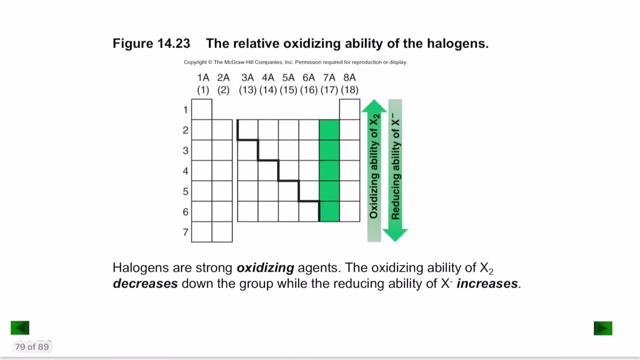 iodine is the least reactive halogen. Next, let's talk about the relative oxidizing ability. So as you go down the group, there is a decrease in the oxidizing ability of the halogen gas and an increase in the reducing ability of the halide ion. 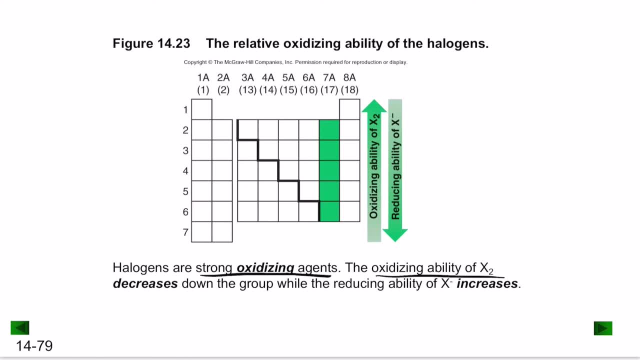 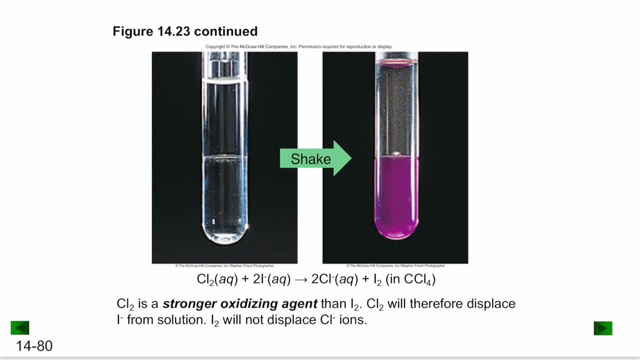 So halogens are generally strong oxidizing agents, So the oxidizing ability of the halogen decreases down the group, while the reducing ability of the halide ion increases. Now, when you mix chlorine and iodine in water and mix them together Rather, that results in the formation of iodine I2 in CCL4.. 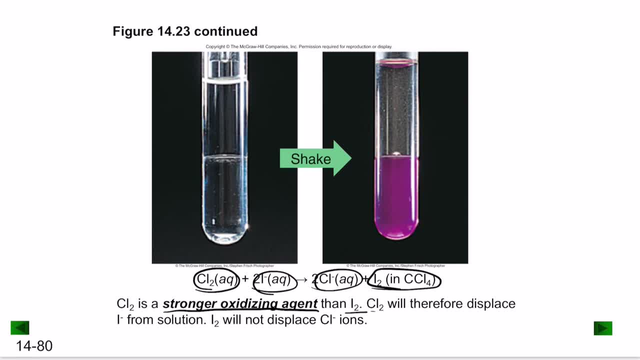 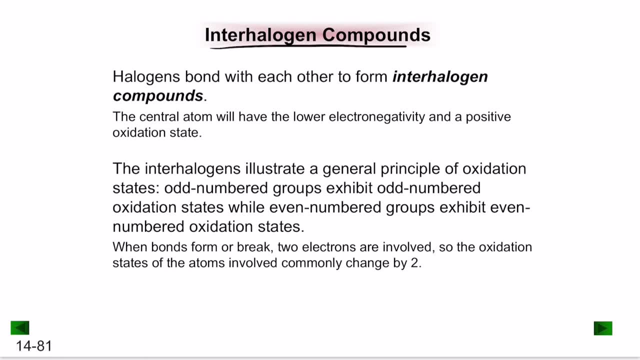 So this chlorine is generally a strong oxidizing agent than iodine. So chlorine will therefore displace iodine from the solution and will result in the formation of iodine. Next let's talk about interhalogen compounds. Interhalogen compounds are the compounds that bond with each other to form interhalogen. 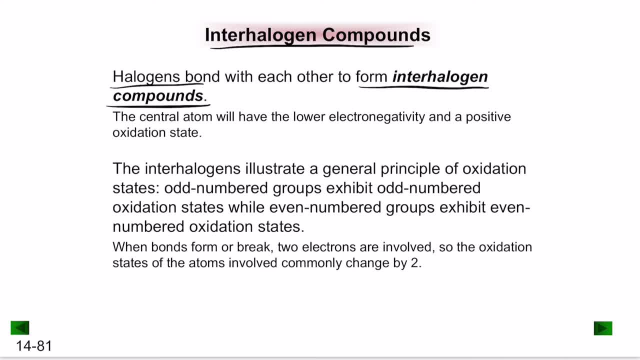 compounds, So for example chlorine with iodine, fluorine with iodine. things like these are generally called interhalogen compounds. So they generally illustrate a general principle of oxidation states: That the odd number groups exhibit odd numbered oxidation states, while the even numbered 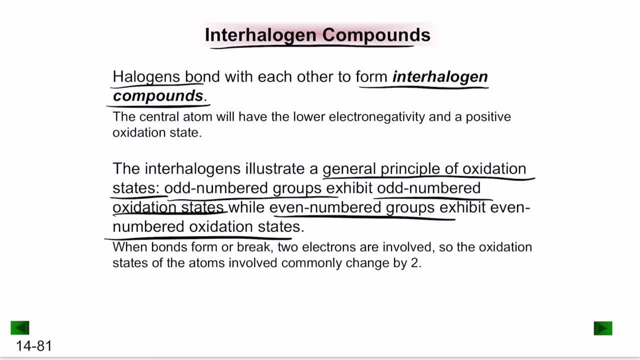 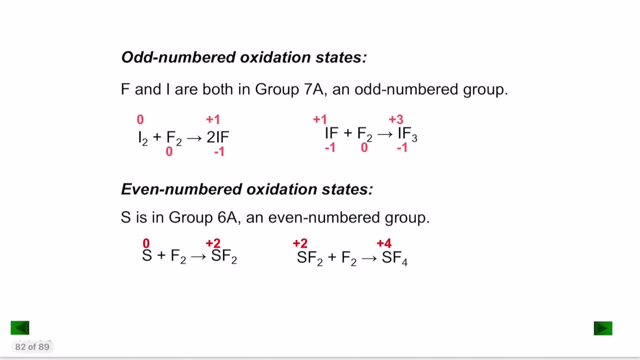 groups exhibit the even numbered oxidation states. So when the bonds break and form, there are two electrons involved. So the oxidation state of the atoms involved commonly changes by two. So let's take a simple example of iodine and fluorine. Notice that both have a zero oxidation number, but when they mix together they result in: 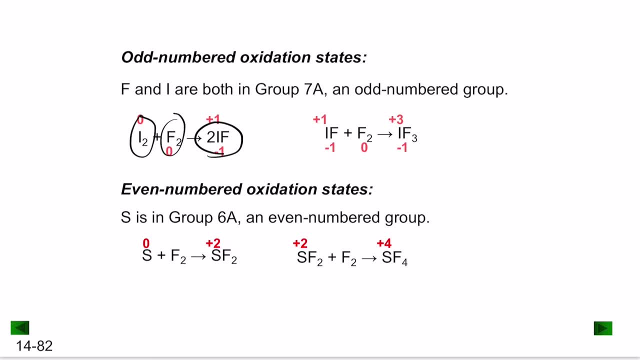 the formation of plus one minus one oxidation number. So this is the idea behind an odd numbered group. When you take a look at an even numbered group where you have sulfur and fluorine, Sulfur results in the formation of plus two, and so an even number will always bond with. 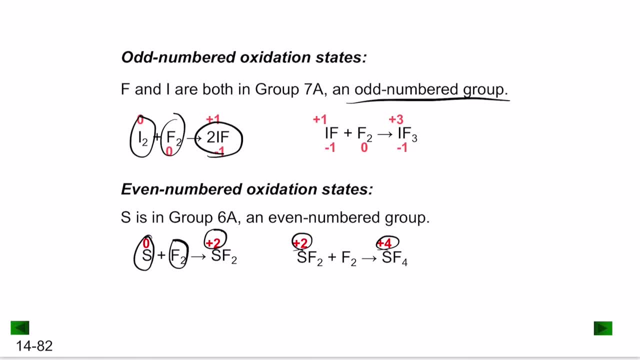 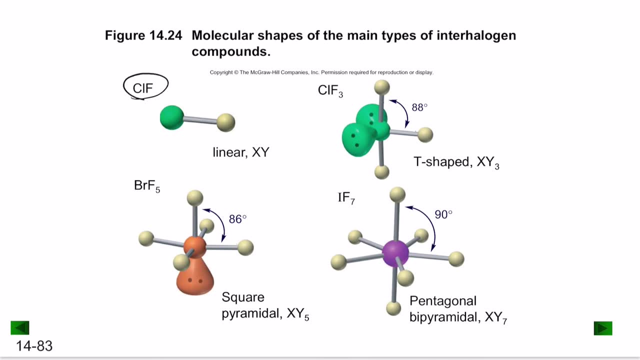 an even numbered one. An odd number will always form a bond with an odd numbered one. Now these are some of the molecular shapes of different interhalogen compounds. For example, CLF is a linear structure, CLF3 is a T-shaped structure, BRF5 is a square. 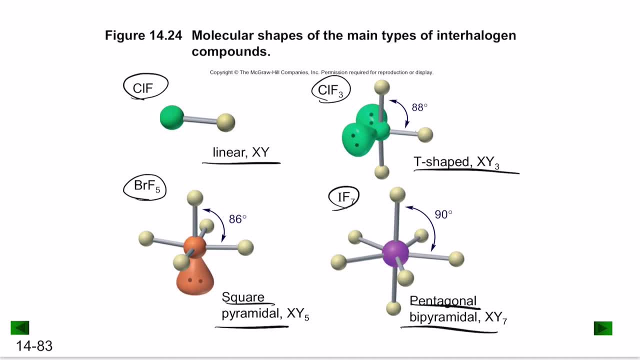 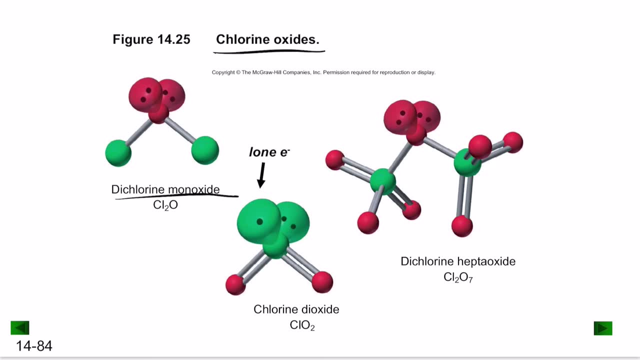 pyramidal structure and IF7 is a pentagonal bipyramidal structure. Now let's look at cloning Clorine oxide. so these are some of the chlorine oxides, so dichlorine monoxide, chlorine dioxide and dichlorine heptoxide. 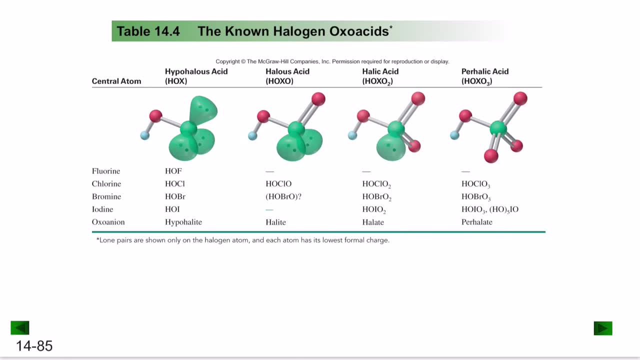 So these are some of the known halogen acids. So halogen acids are generally arranged based on the amount of oxygen that is present. If there is one oxygen, we call it a hypohalous acid. For example, HOF is hypofluorous acid, HOCl is hydro hypochlorous acid- hypobromous acid. 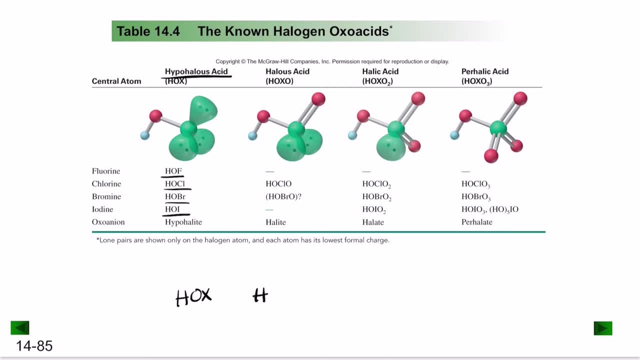 and hypoiodous acid. If there are two oxygens, then we call that a halous acid. So an example of this would be: if you take HOClO, then that would be called chlorous acid. HOClO2 is halic acid. 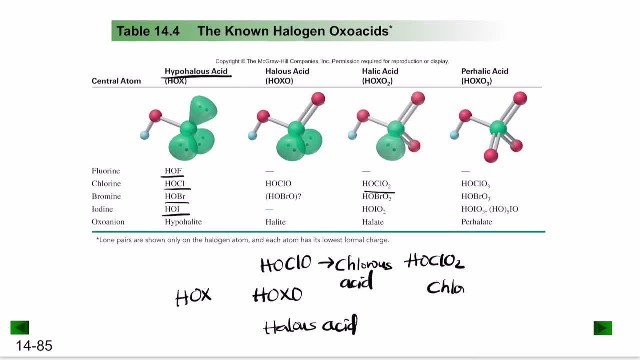 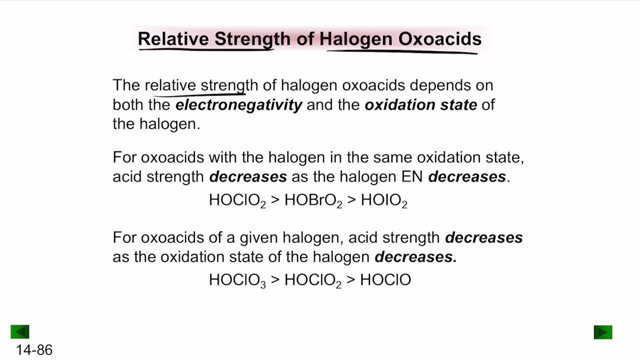 This is Cl, so we can call this chloric acid, And you have HOClO3. that results in the formation of perhalic acid. Now let's talk about the relative strength of the hydrogen halogen oxo acids. So the relative strength of the halo acids generally depends on both electron activity. 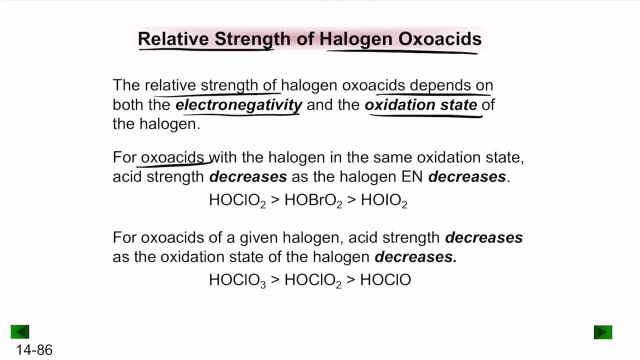 and the oxidation state of the halogen. So for oxo acids with the halogen in the same oxidation state, acid strength generally decreases as the halogen electro negativity decreases, Which basically means chlorine has the highest one, with iodine having the least one provided 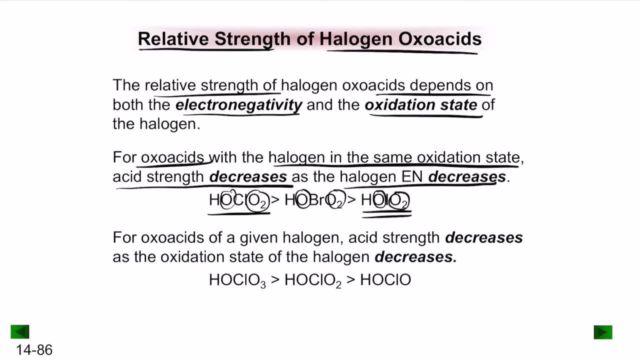 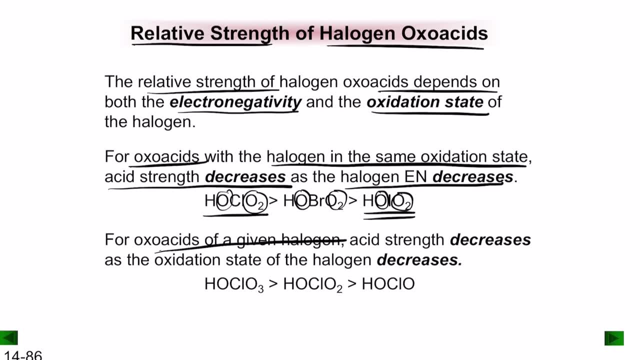 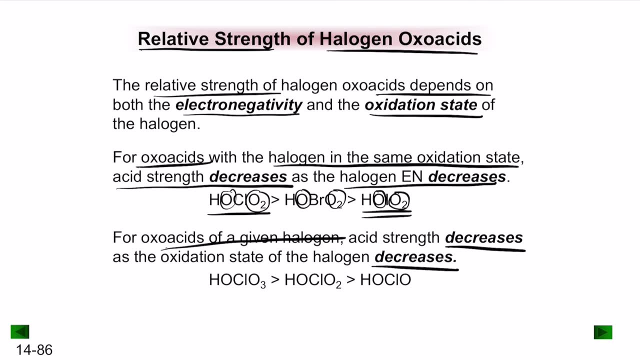 they have the same number of oxygens in all of them. Now, if you are talking about different acids with different number of oxygens, So for our oxo acids, with the halogen given, halogen acid strength generally decreases as the oxidation strength state of the halogen generally decreases. 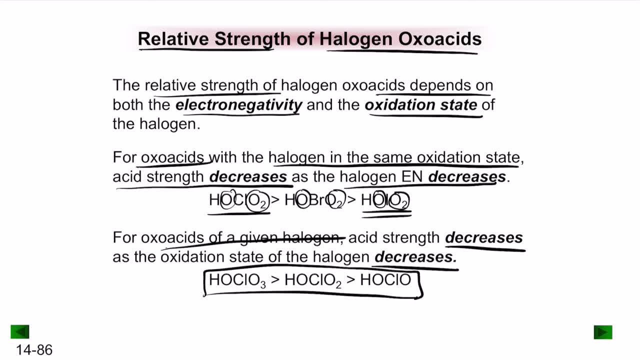 So HOClO3 is greater than HOClO2.. So the halogen free periods have the same number of musician greater than HOClO. So the more the number of oxygens, the stronger the acid, provided all of them have the same halogen in them. So finally, let's go to group 8 elements, the noble gases. So 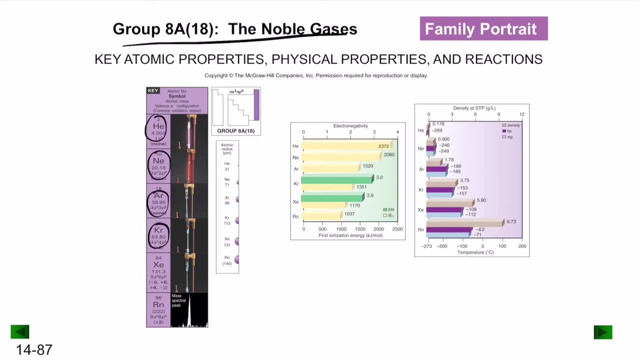 these are helium, neon, argon, krypton, xenon and radon. Now these generally have the electronic configuration NS2NP6.. It's more commonly known as the noble gases or inert gases. So the name inert gases is not the right name. The reason mainly is because, even though all elements do,